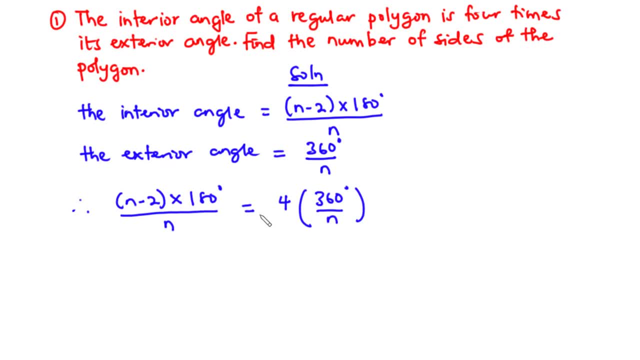 the number of sides, that is n. Now, at this point, we can choose to cross-multiply or we can choose to cancel out n. n goes into itself once, n goes here once. Therefore, we have n-2, all times. 180, equals 4 times. 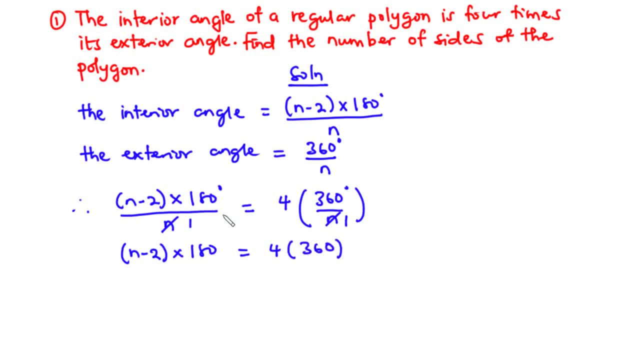 360.. Now, if you choose to cross-multiply, you will definitely arrive at the same expression or the same equation. Now let's multiply 180 degrees across, So we have 180n minus 360, and that is equal to 4 times 360 is 1440.. Now we transpose negative 360 to the right hand side, We have 180n equals. 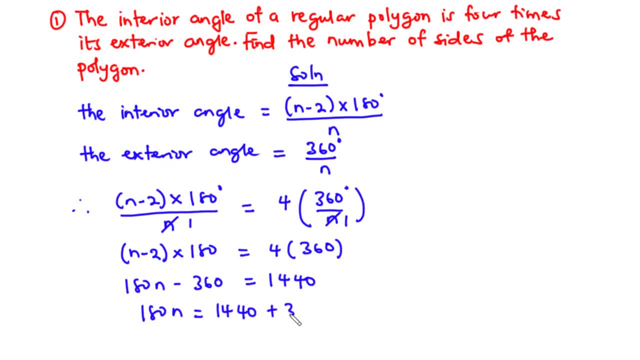 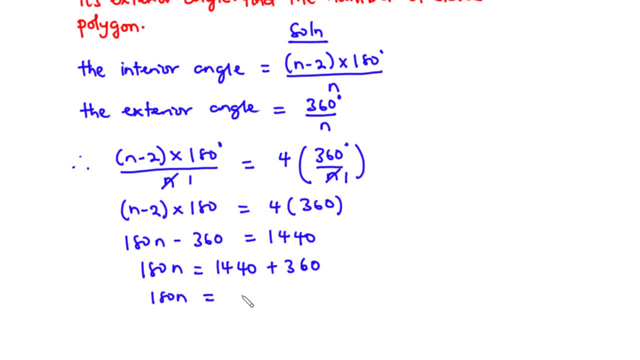 1440 plus 360. And that becomes 180n equals 1440 plus 360 is equal to 1800.. Since we want to find the value of n, we divide through by 180. And then we have n to be 10.. 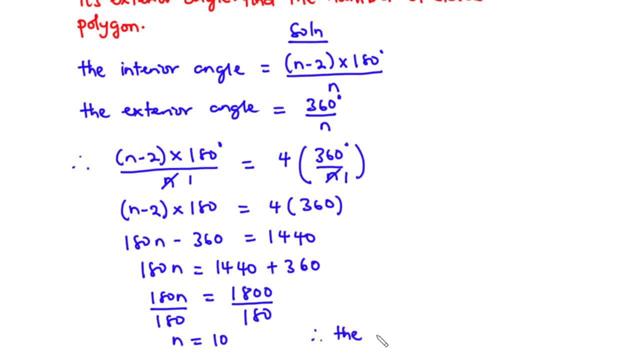 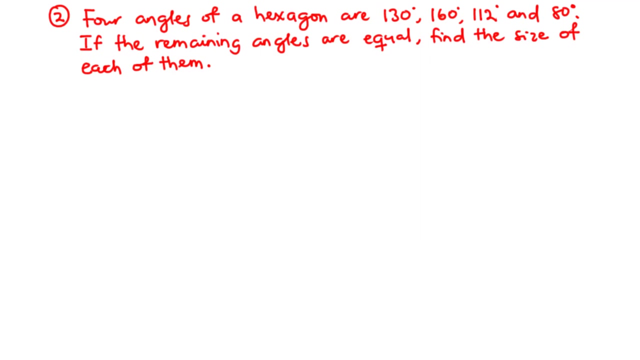 Therefore, the polygon has 10 sides. Now let's solve the next example or the next question. Now to example 2.. Four angles of a hexagon are 130 degrees, 160 degrees, 112 degrees and 80 degrees. Now if 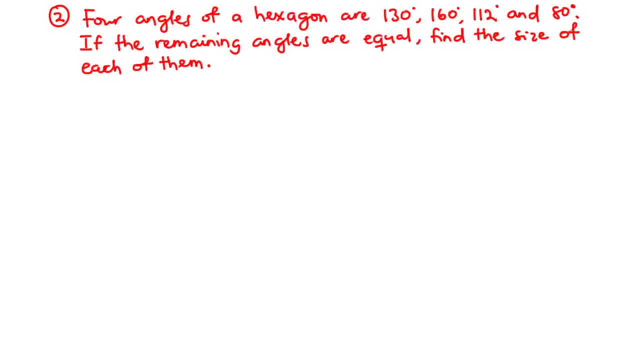 If the remaining angles are equal, find the size of each of them. Now for this question. we are given four angles of a hexagon, And we know that a hexagon is a polygon with six sides. If four of the angles are given, then it means that we have two unknown angles. 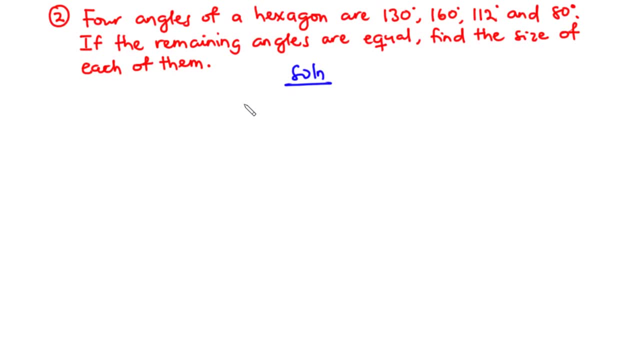 And also from the question. we are being told that the two unknown angles are equal. Therefore, If a hexagon has six sides, Then for the unknown angles, let x represent both angles or the value of both angles. Therefore, for the six angles, we have 130 degrees, 160 degrees. 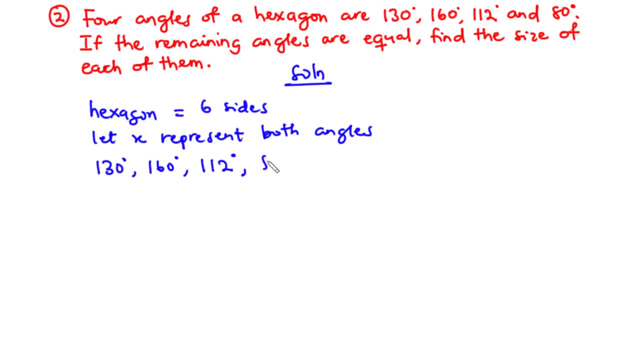 112 degrees, 80 degrees, x degrees and x degrees. So these are the six angles for the hexagon in question. Now to find the size of each of them, that is, the x angles, We need to find the sum of interior angles of this hexagon. 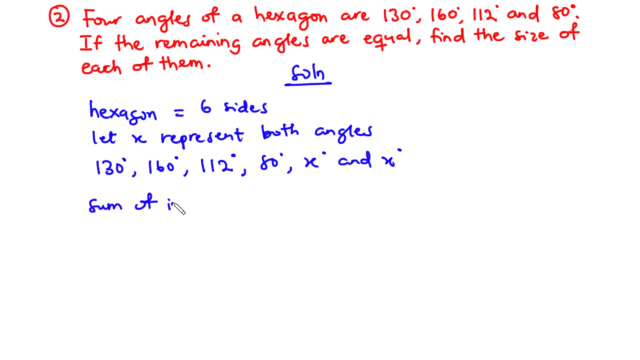 So the sum of interior angles Of the hexagon Is given by n minus 2 times 180 degrees. And since a hexagon has six sides, we substitute six in place of n, So that we have 6 minus 2 times 180.. 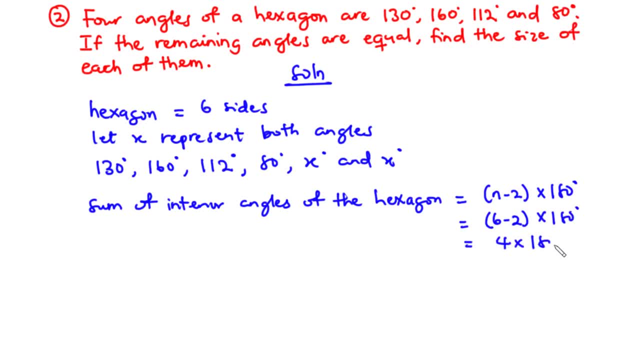 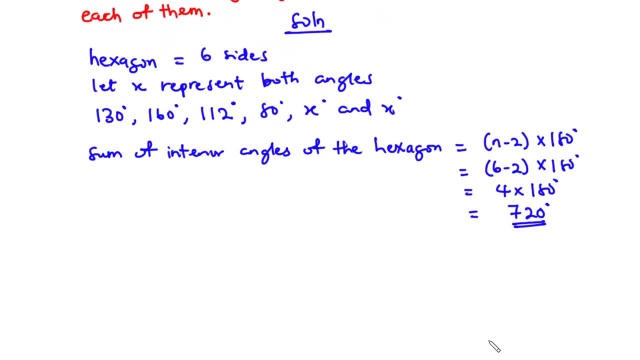 We have 4 times 180.. And that is equal to 720 degrees. Now to find the value of x, we need to add up all these values and equate to 720.. Therefore, we have 130 plus 160 plus 112 plus 80 plus x plus x equals 720. 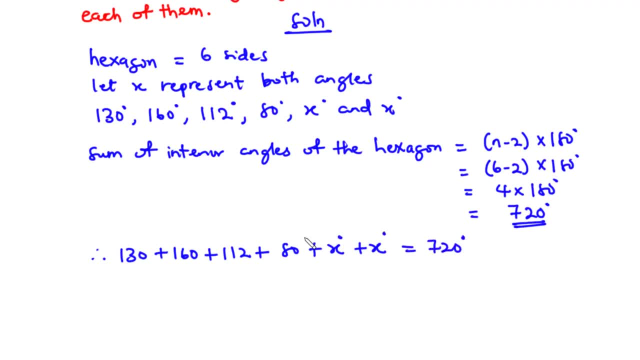 So 130 plus 160 plus 112 plus 80 gives 482.. And then x plus x we have 2x. So we transpose this value to the right-hand side, We have 2x equals 720 minus 482..